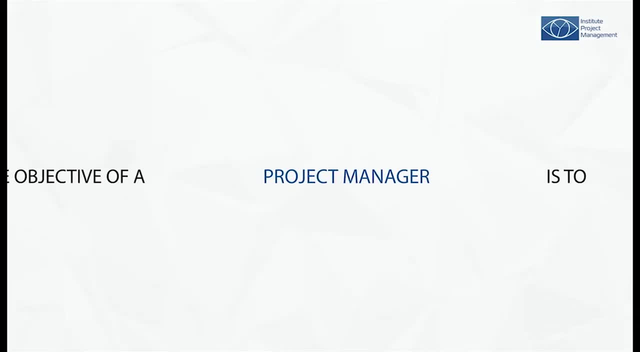 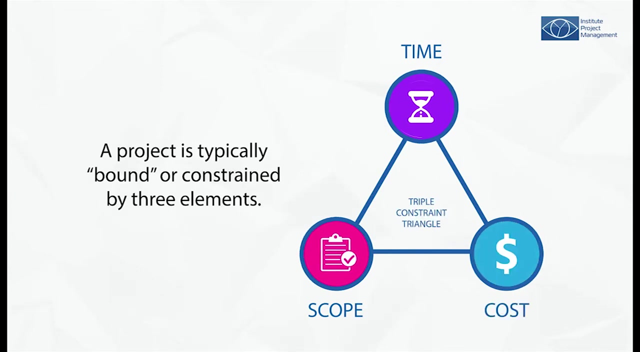 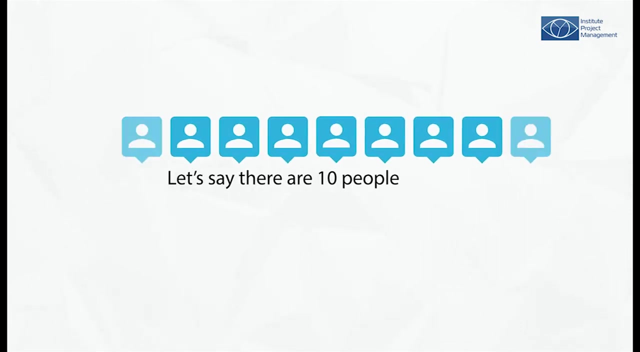 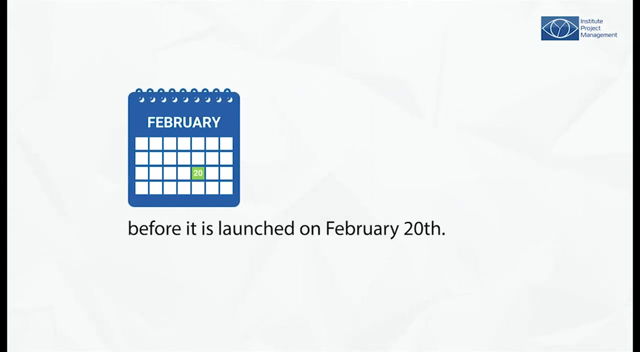 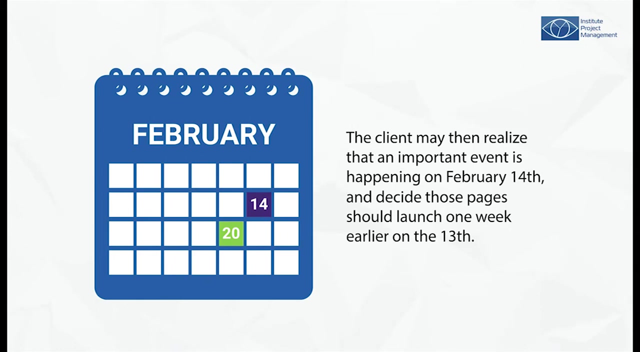 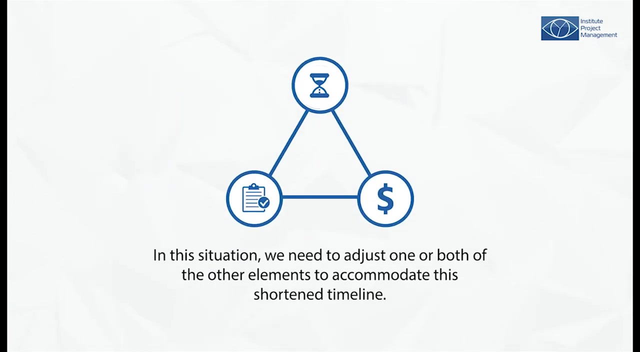 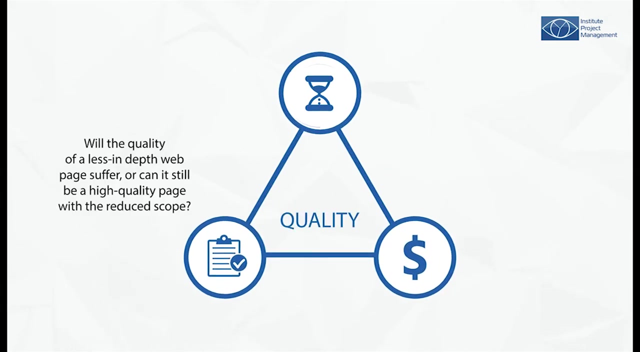 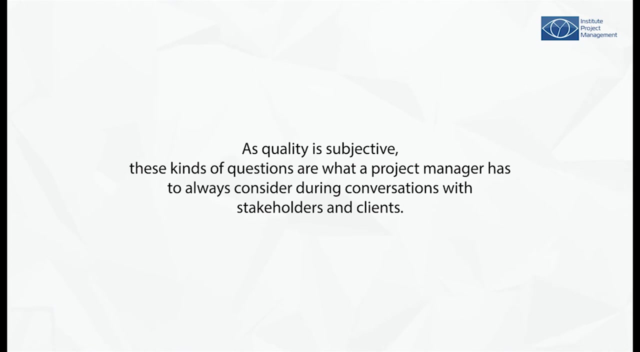 Library betrayer. We have this application with a ton of information because we are a buraya, We are the company of doctors in the客. Thank you, Thank you, Thank you. 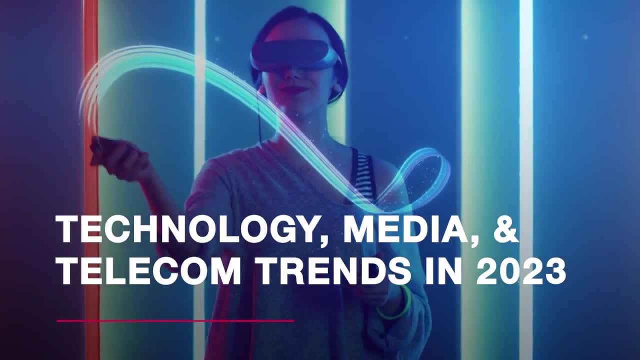 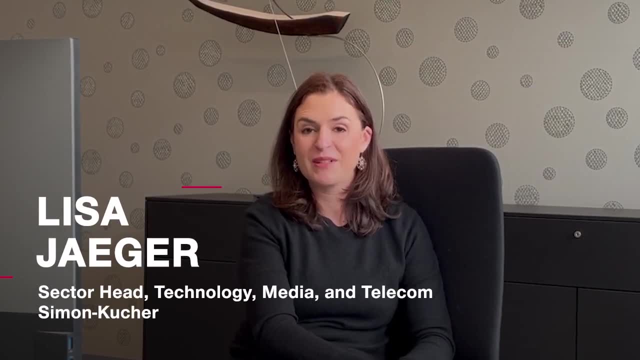 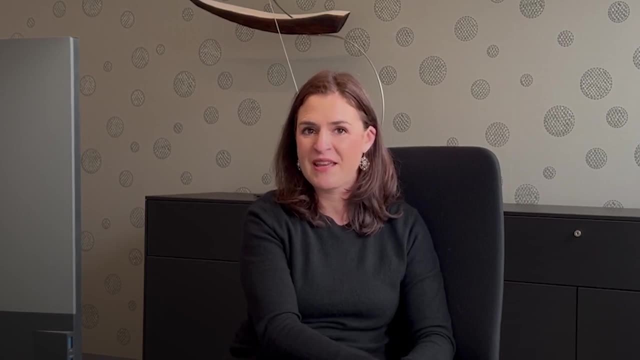 Tech, media and telco companies were some of the last to be hit by the economic downturn, But no company is immune to things such as increasing interest rates and therefore money getting more expensive, impacts on company valuations and reactions on stock markets. But one thing all. 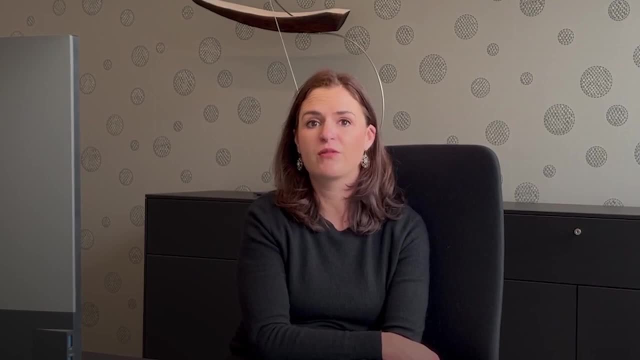 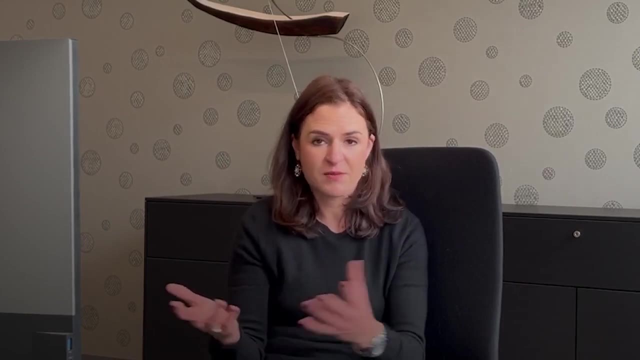 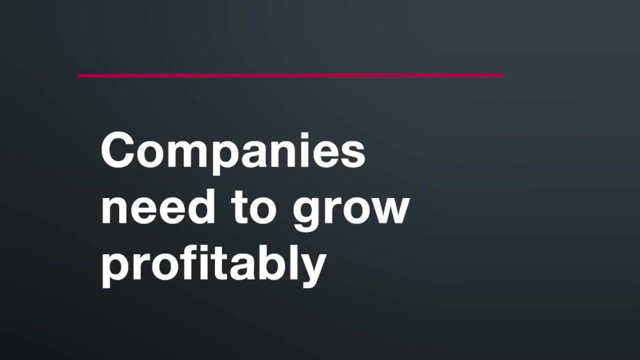 of these companies have in common is that they need to increase prices. Why? Because they have to pay higher wages, they have higher costs and if they don't increase prices, it's pure margin loss. Companies need to grow profitably In 2023, acquiring new customers will not be the only. 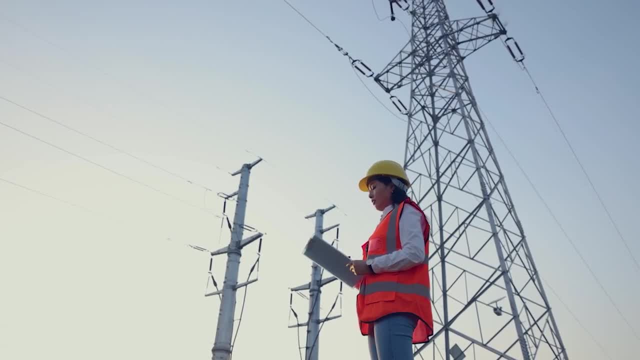 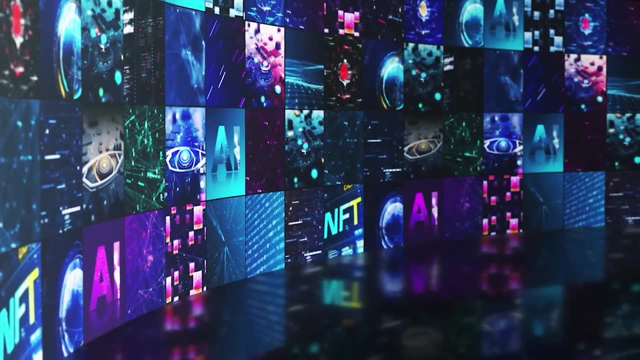 source of growth. For many companies, it's actually more expensive to acquire new customers than maintaining the existing customers, And therefore growth needs to come from monitoring and monitoring of the market, And that's why we have to pay higher wages. It is due to the어지the number of customers that buy using the condition and not the.